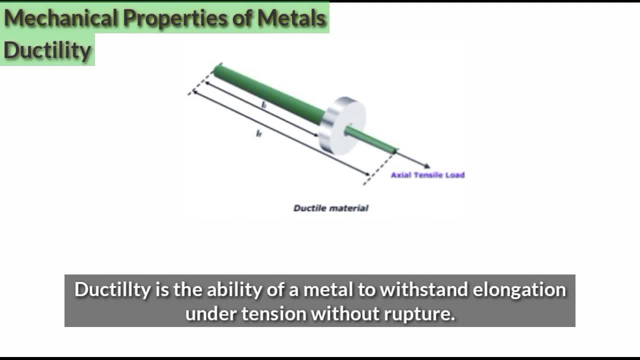 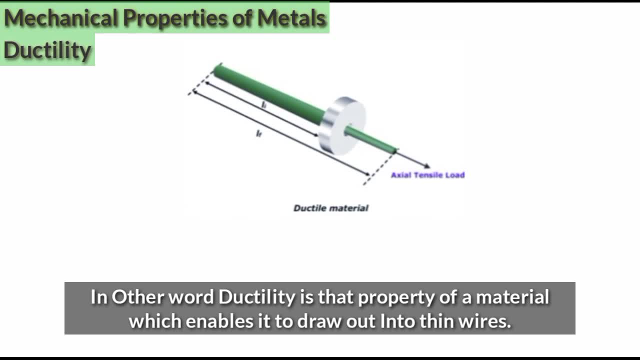 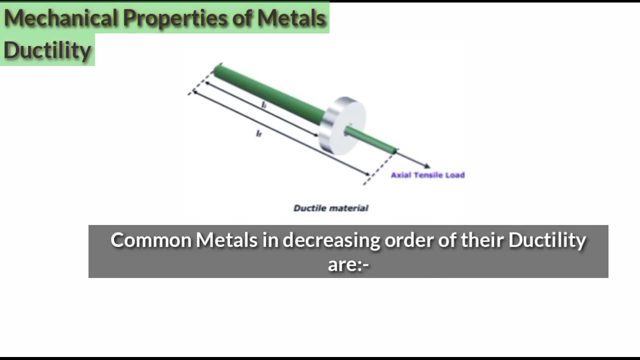 So ductility is the ability of a metal to withstand elongation under tension without rupture, Or, in other words, ductility is the property of material which enables it to draw out into thin wire. Common metals, in decreasing order of their ductility are gold, silver, platinum, iron. 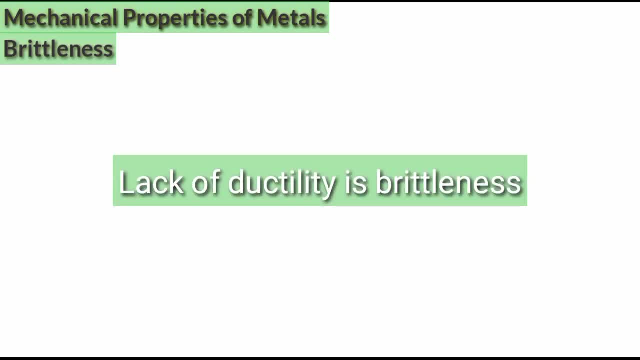 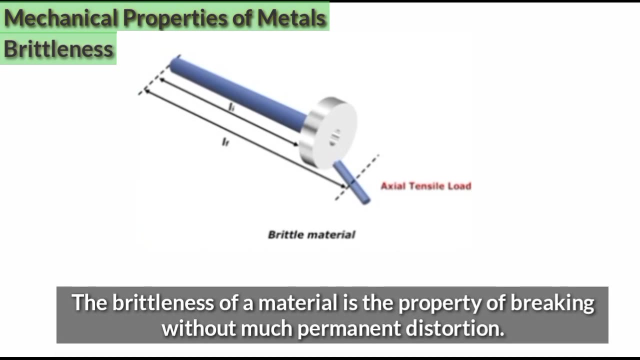 Brittleness. Lack of ductility is brittleness. To understand brittleness, let's also take another metallic bar. This metallic bar, when subjected to axial tensile load, we notice that bar does not elongate and fail. So we can say that brittleness of a metal is the property of brittleness, without much. 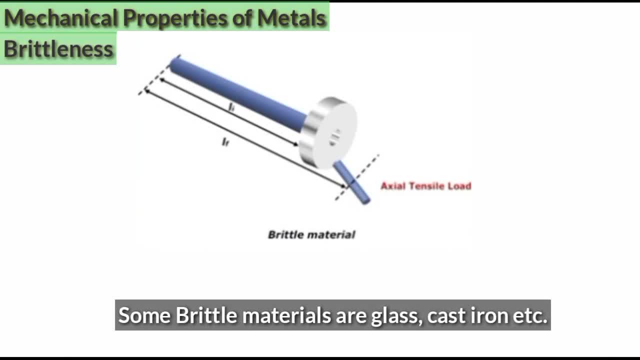 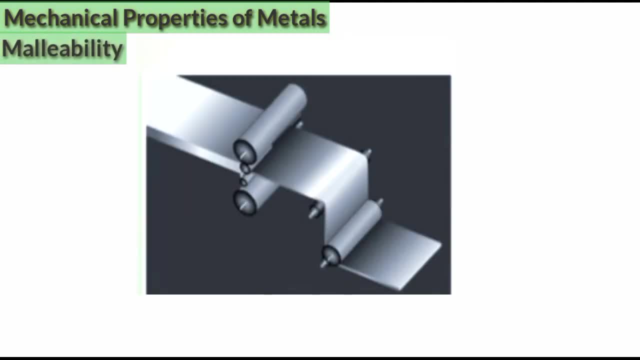 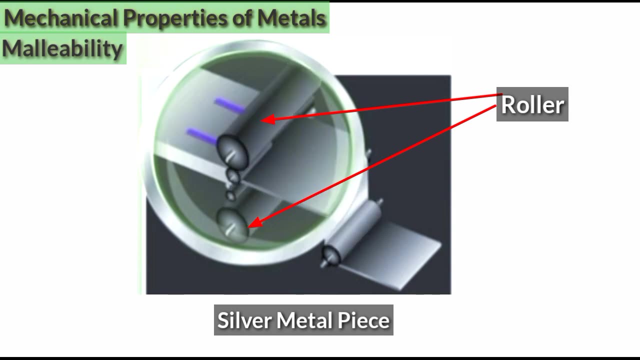 permanent distortion. Some brittle metals are glass, cast iron, etc. Malleability. To understand malleability, let's take an example of a silver metal piece. When we pass this silver metal piece through a roller, it gets deformed into a thin sheet. 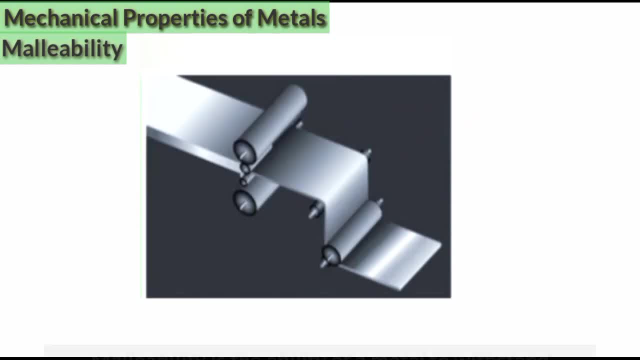 of a metal due to the compressive load applied by the roller. So we can say that brittleness of a metal is the property of brittleness, without much permanent distortion. So malleability is the ability of a metal to withstand deformation under compression. 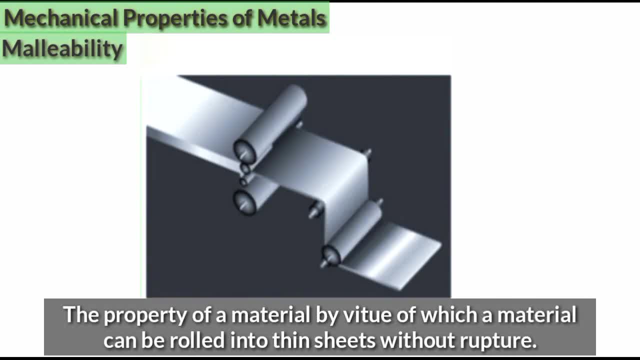 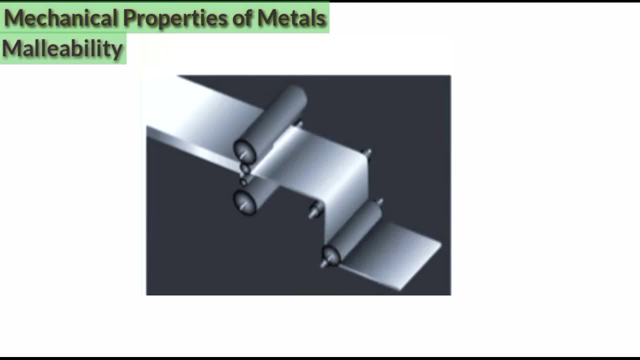 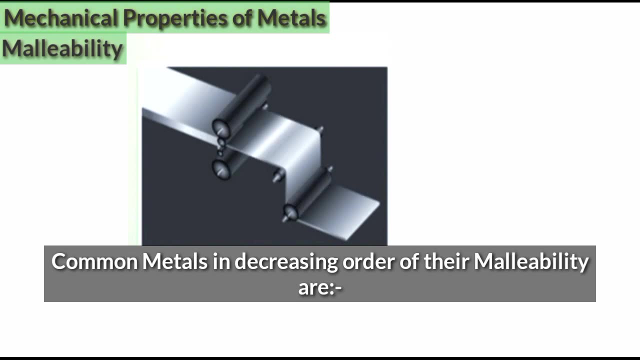 without rupture, Or in other words, it is the property of a metal by virtue of which a metal can be rolled out into a sheet without rupture. This property generally increases with the increase of the temperature. Common metals in decreasing order of malleability are gold, silver, copper and aluminum. 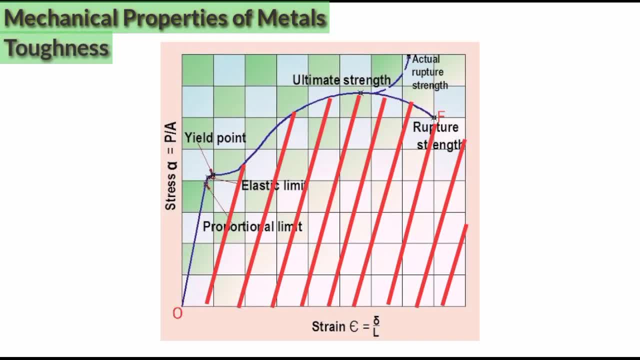 Toughness. To understand toughness, let's take an example of a metal. To understand toughness, let's take a stress-strain curve for ductile material In figure from 0.02, a shaded portion indicates energy absorption capacity of a material. before. 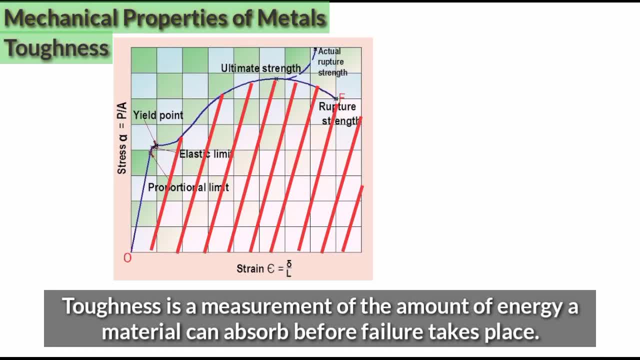 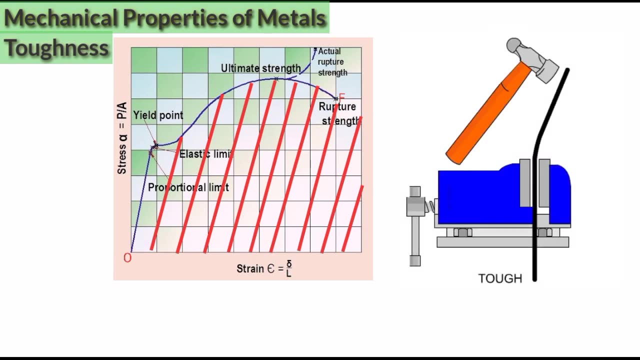 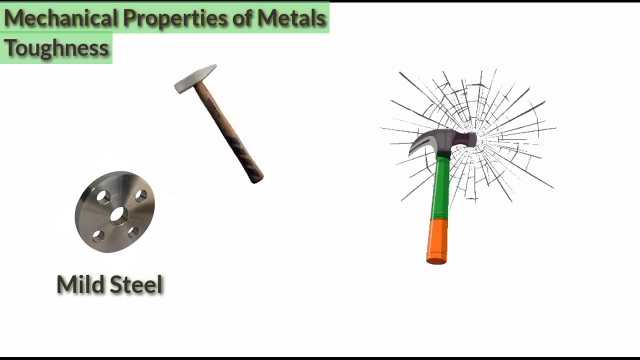 fracture. So toughness is the measurement of the amount of energy a material can absorb before failure takes place. The toughness of a metal is expressed as an energy absorber. Toughness is related to impact strength, That is, resistance to shock. For example, if a load is suddenly applied to a piece of mild steel and then to a piece